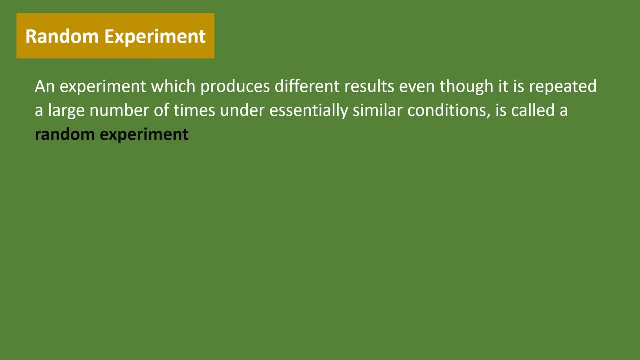 Random experiment repeated large number of times under similar condition and it will give different result. Example 1: tossing of a fair coin. Tossing of a coin. there is two possibilities: head and tail Tossing of a coin or random experiment Throwing of a balanced dice. It has six possible outcomes. There are random experiment. 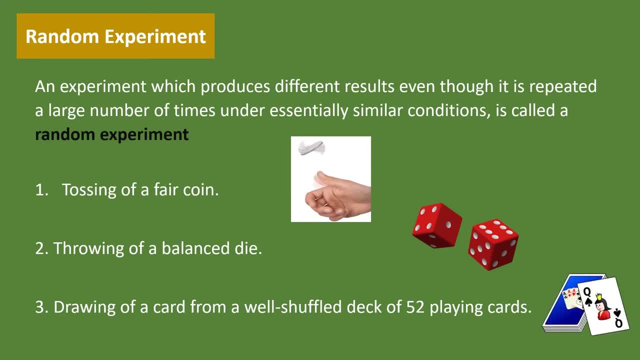 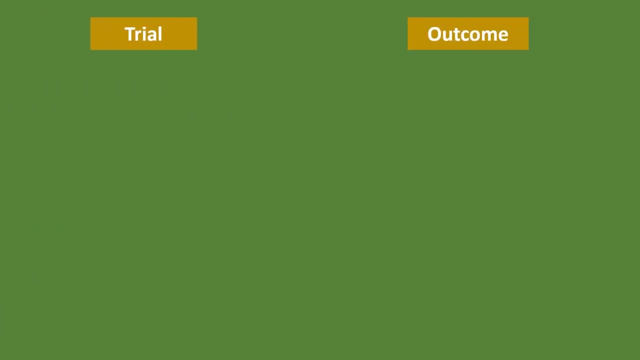 Drawing of a card from a well-shuffled desk of 52 playing cards. There have 52 possibilities. There are also called a random experiment. A single performance of an experiment is called a trial. The result obtained from an experiment or a trial is called a outcome. Tossing of a fair coin. example: Tossing a coin: two possible. 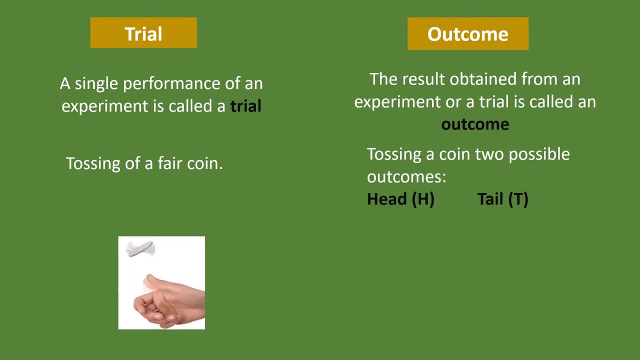 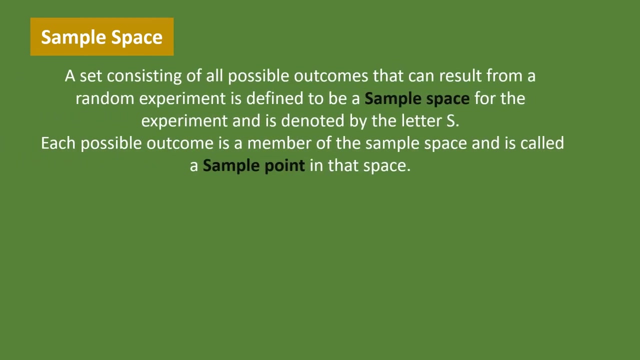 outcomes: head and tails. Tossing of a coin are called two possible outcomes. There are TROIL. HEAD and TAILS are outcomes. Sample Space- A set consisting of all possible outcomes that can result from a random experiment is defined to be a sample space for the experiment. 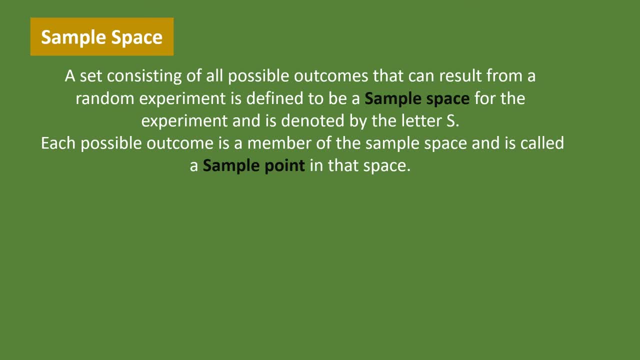 and it denoted by the letter S: The possible. all possible outcomes are called sample space. Each possible outcome is a member of the sample space and it called a sample point in the space. Each possible outcome are called sample in sample space are called sample point. 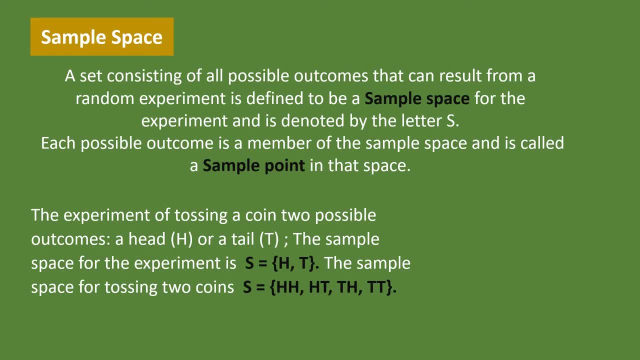 Example: the experiment of tossing of two possible outcomes, a head and tail. The sample space for the experiment is head and tail. The sample space for tossing two coins S is equal to head-head, head-tail, tail-head and tail-tail.